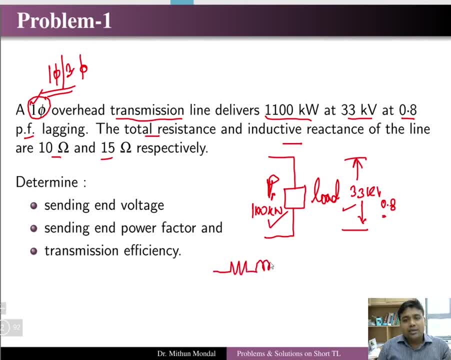 we know that in the short transmission line we will neglect the shunt capacitance. So we have been given the values of the resistance, that is, 10 ohm, and 15 ohm is the value of the reactance, and a load is connected at the receiving end and this is our. 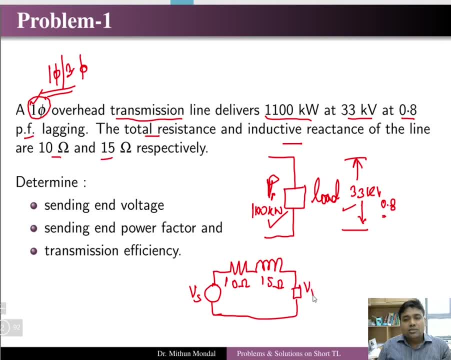 sending end voltage. So, since this is a single phase transmission system, we need not to change anything. We will just use the data whatever is given. Now we have to obtain what is the sending end voltage, what is the power factor of the sending end and what is the transmission. 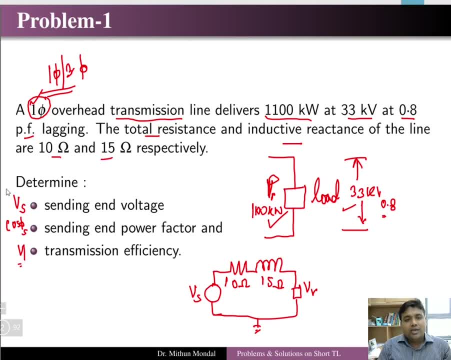 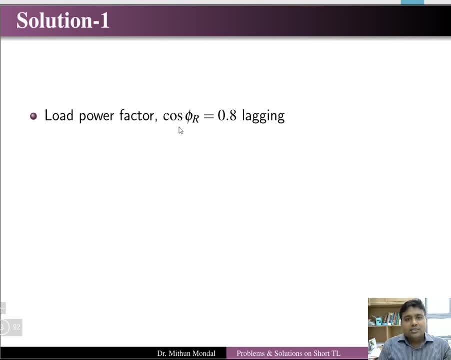 efficiency. So these particular things we have to obtain from the problem number 1.. Now let us see So, given condition is that the power factor of the receiving end is 0.8 and the total line impedance is given to be 10 plus j15, that is, r plus jxx. 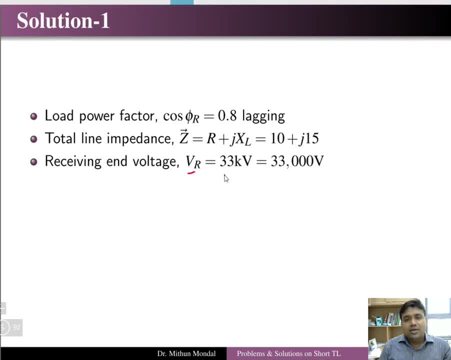 cell, Then the receiving voltage is 33 kV, since it is a single phase. so this is basically the phase voltage. Now you can obtain the line current. we know the formula for power is equal to V phase. I phase into cos phi. From here we have been given the value of power and we have been given 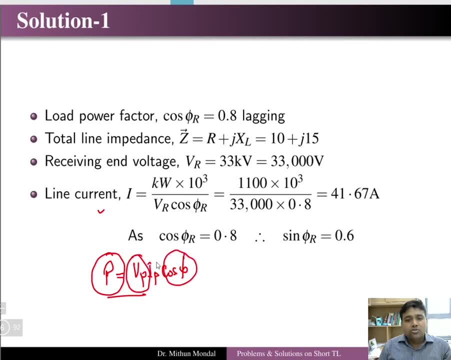 the value of the voltage and the power factor. So the only unknown is the current. So we can obtain that current, which is the phase current, or equal to the line current, because it is a single phase quantity that will give you 41.67 ampere. Also, we know that cos phi r, that is the 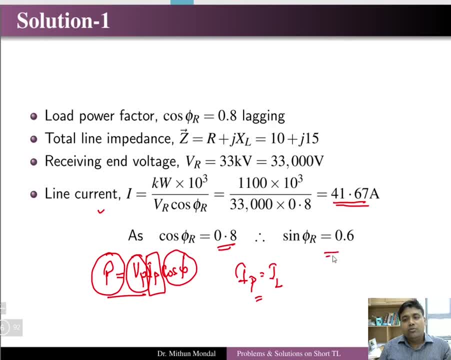 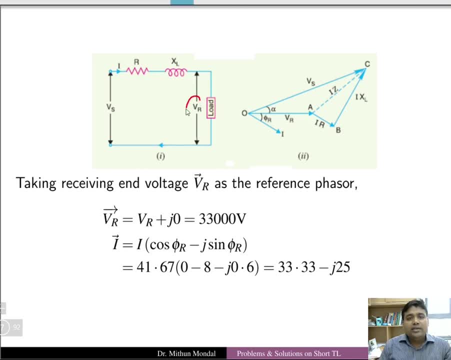 receiving and power factor is 0.8, so sin phi r value will be 0.6.. Now we will start from the receiving end quantity, that is, we will take the receiving end quantity as the reference. So if we take the receiving end quantity as the reference, it means it will be on the 0 axis. 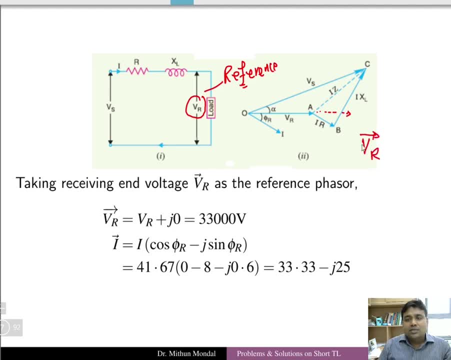 So receiving end vector would be equal to the receiving end magnitude with an angle of 0 degree. Then other quantities we can write, we can obtain based on the reference quantity. So we have been given that the 33 kV is the receiving end voltage. Then what is the current flowing in this circuit? 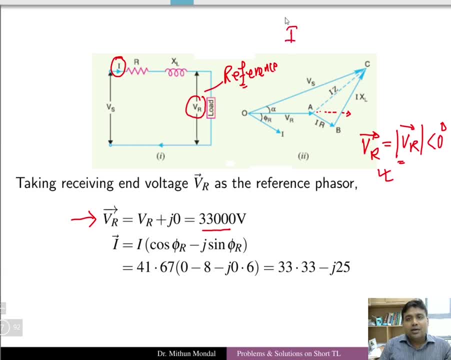 So the current flowing is basically the current vector, is basically the magnitude of the current and the angle of minus phi, because you have been given the line current. So the current flowing is the lagging power factor condition. So we have obtained the value of cos phi r and sin phi r and we 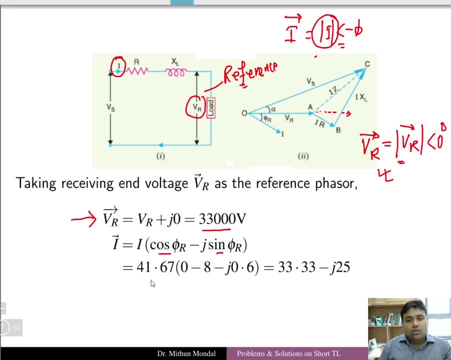 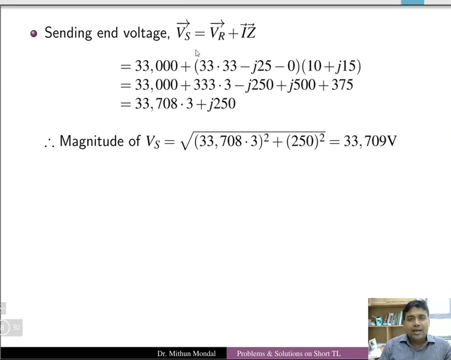 have also obtained the magnitude of the current. So the value of the magnitude is 41.67 and the cos phi r and sin phi r component we have calculated. So this is the current vector which we have obtained. Next we have to obtain the sending end voltage. We know that we can write a. 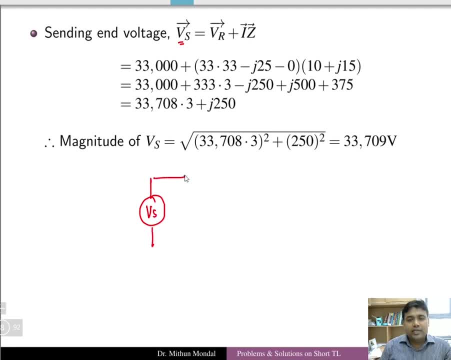 KVL equation in this loop. So sending end voltage is basically: so this is the total impedance of the line and this is equal to the receiving end voltage of the line. So this circuit, and here you have the flowing, the current, I. So if we write the KVL equation, what you will get? the sending end. 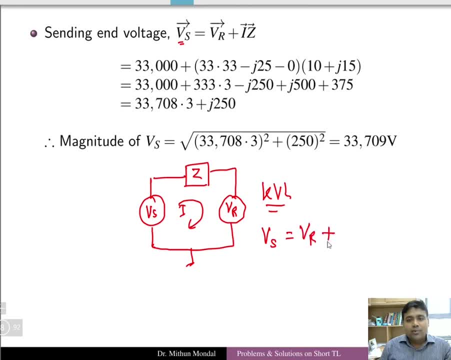 voltage is equal to receiving end voltage plus the current multiplied with the impedance. Now these are all vector quantities. So we will take all as vector quantities and then we will substitute the value of Vr, current and the impedance. So after substituting we are getting this value of sending. 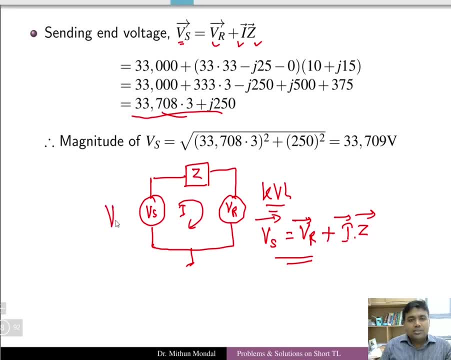 end voltage. So the magnitude of the sending end voltage we have to calculate. So it is basically, under root, the real square plus the imaginary square. So the real quantity is 33708.3 and the voltage is 33709.3.. So you are getting 33709 volt as the sending end voltage. Now we have to determine. 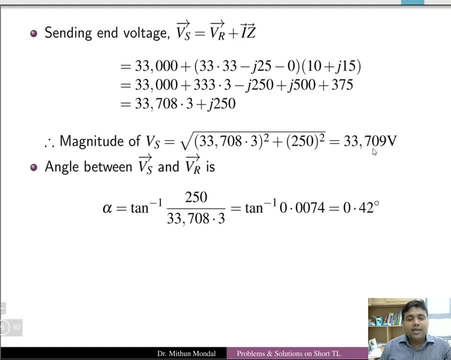 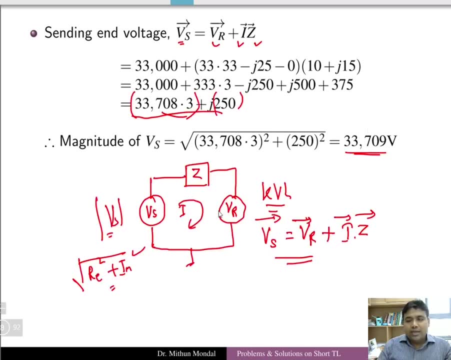 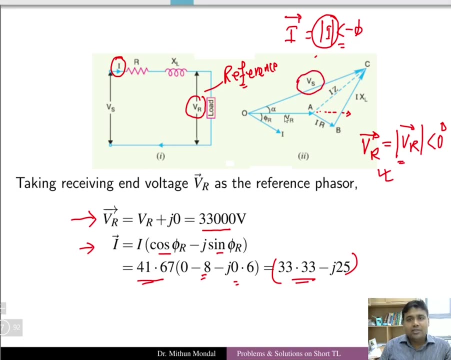 in the next case, what is the sending end power factor? that is cos of phi s. So before that, we will see that the value of phi s, that is, the sending end power factor, is the angle between the voltage and the current. So phi s will be equal to the value of phi s, which is the 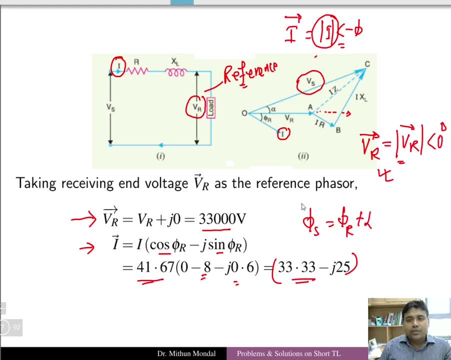 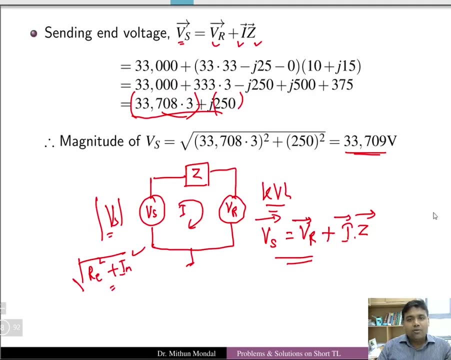 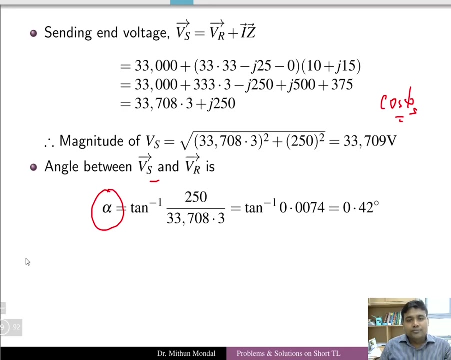 사랑 that we got earlier as respect to phi r plus alpha. Phi r is basically the angle between the receiving end voltage and the current, and alpha is the angle between Vr and Vs. So we have obtained both Vr and Vs, so from which we can calculate what is the value. 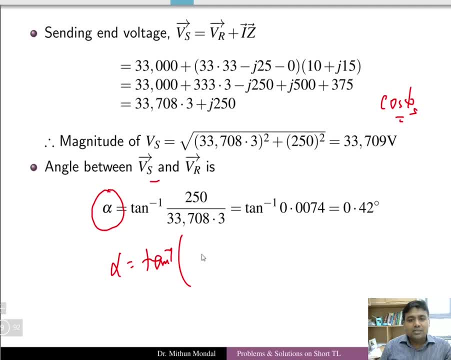 of alpha. So value of alpha is basically viendo 10 inverse. That is the angle between of alpha we have of the magnitude of the Vs. So here you have the imaginary quantity Q and here you have the real quantity P. So divide the Q by P, So this, you will get the value of alpha, which is equal to. 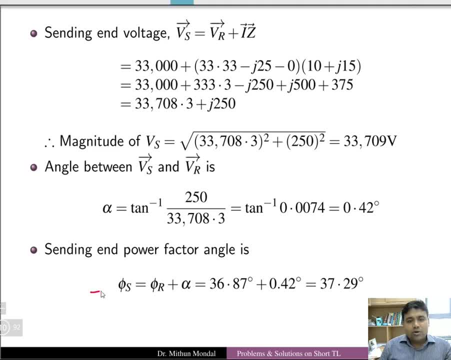 0.42.. Then the sending and power factor phi s will be equal to phi r plus alpha. So phi r is basically the power factor angle of the receiving side plus 0.42. that is we have obtained here. So it is 37.29.. So this angle plus phi r plus alpha, you will get the value of phi s. Next, what is the? 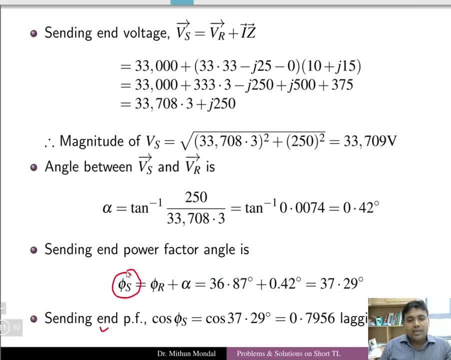 sending and power factor. Now you have obtained the power factor angle, So cos phi s will give you the sending and power factor, which is coming to be 0.7956 because the angle is 37.29.. So cos of 37.95 will be 0.7956.. So this is the value of phi r plus alpha. So this is the value of phi r. 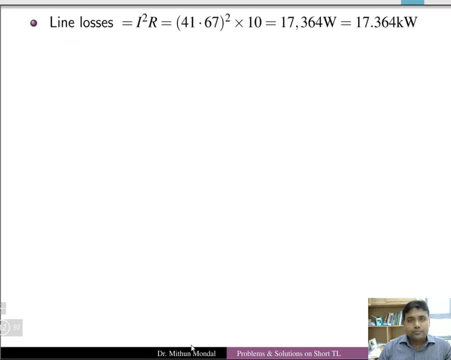 and 37.29 will give 0.7956.. Now we have to determine what is the efficiency. So efficiency is basically power output by power input, and input power can be written as power output plus losses. So we have to calculate what is the total loss in the transmission line. So here you will get. 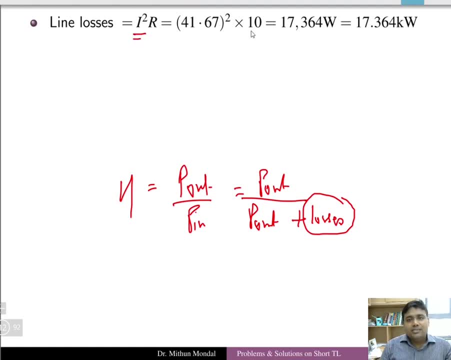 I square r as the loss of phi, r plus alpha. So this is the total loss in the transmission line Where the resistance is given to be 10 ohms and the magnitude of the current is 41.67.. So you will get 17.364 kilowatt as the line losses And the power output is basically is given in the question. 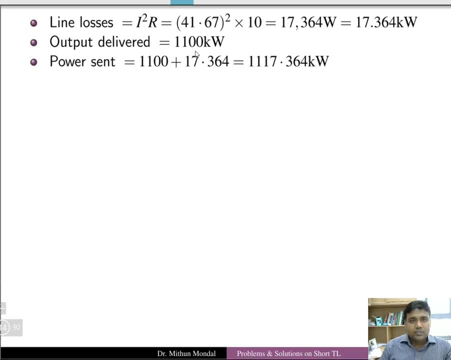 as 1100 kilowatt, Then the power sent, because you have power input, is equal to power output plus losses. So power output is 1100 kilowatt plus the losses. you have calculated as 17.364.. So you add it. you. 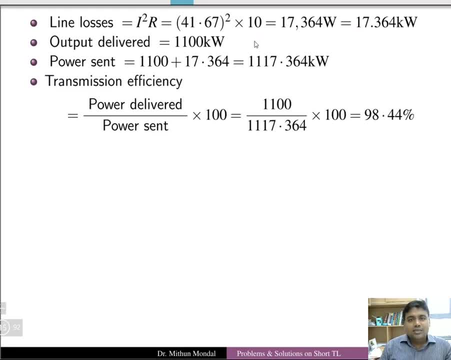 will get the value of power sent as this much. Then it is easy to calculate the transmission efficiency, as power delivered is power output by power input into 100, which gives you 98.44 percent as the transmission efficiency of the line. There is an other way, from the vector diagram, that you can use to calculate this problem of 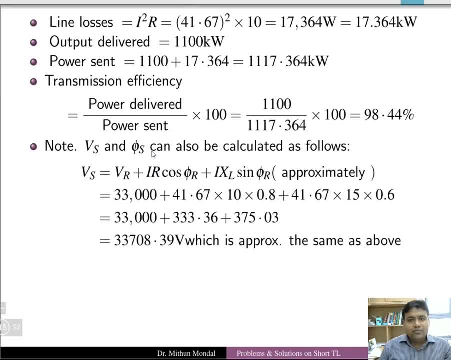 V s and phi s. So directly we know that the formula of V s is this, approximately, which comes from the vector diagram, phasor diagram of the transmission line. So transmission line. So V s is equal to V r plus I r cos phi r plus I x l sin phi r. Please look into the lecture video to 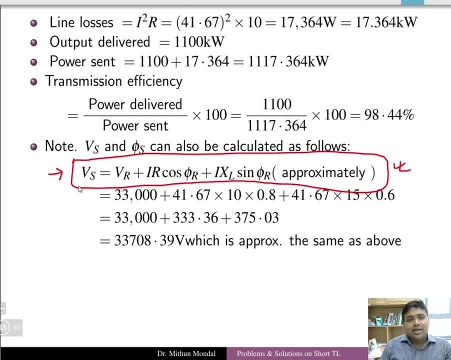 understand where from this formula comes. So we can directly substitute the values of V, r and all the current resistance and reactance, which will get 33708.39, and we will see that it is approximately the same as we have obtained in the previous case. And the value of cos phi s we can again substitute. 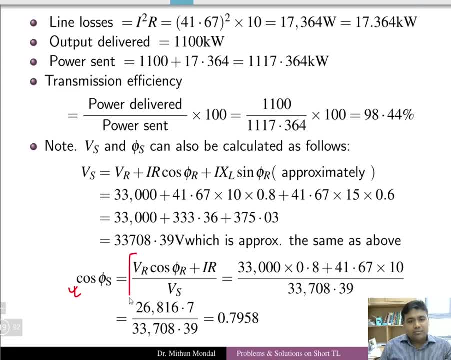 from the values of the phasor diagram. So this cos phi s is equal to this value. V r cos phi r plus I r divided by V? s. So here we are getting a cos phi s is 0.7958, which is approximately equal to 0.8 power factor. So in this way we can solve the problems of short. 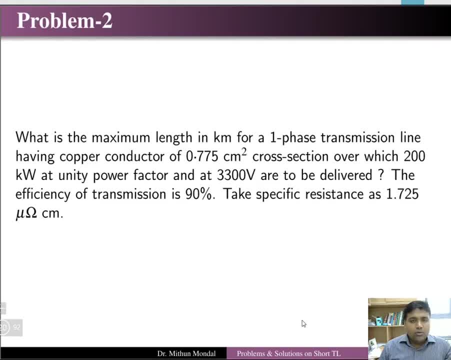 transmission line single phase transmission line. Problem number two is: what is the maximum length in kilometer? that is, we have to calculate the length of the transmission line and the transmission line single phase, which is having a copper conductor of 0.275 centimeter square cross section. 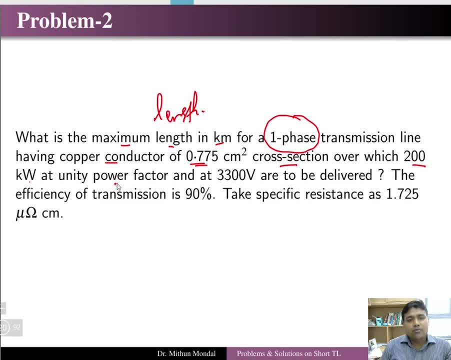 over which 200 kilowatt at unity power factor condition. So basically, the power output is given to be 200 kilowatt, power factor is unity and the voltage is 3300 volt, which is equal to the receiving end voltage. So this is the receiving end. it is equal to cos phi r. 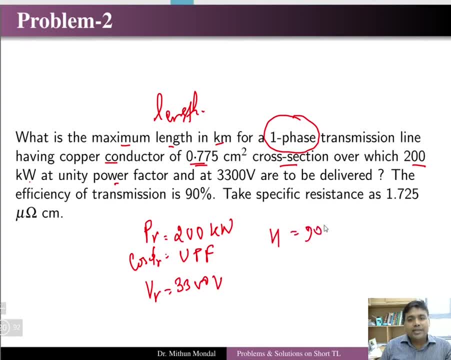 So the efficiency of the transmission is given to be 90 percent and the specific resistance of the material copper is given to be 1.725 micro ohms centimeter. So you have to determine what is the length of the transmission line. What is the length of the transmission line? So let us see. 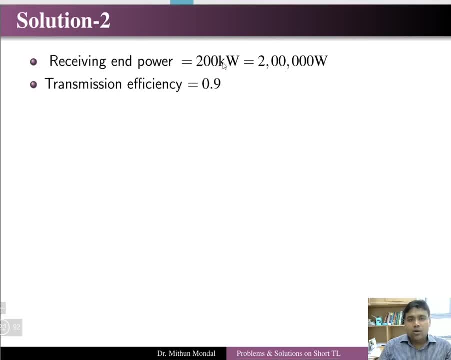 So receiving end power is given to be 200 kilowatt. transmission efficiency is 0.9 and we know from the output by power input. So power output is given, efficiency is given. we can easily calculate what is power input. So power input, that is the sending end power, is this much? Next we can. 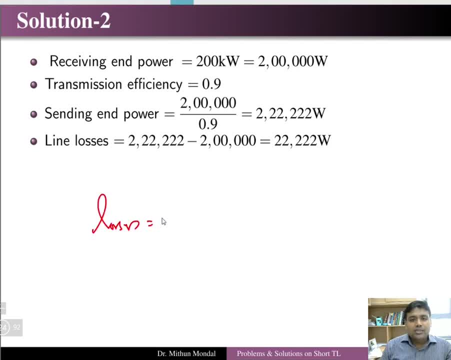 calculate the losses. So losses is basically power input minus power output. So if you subtract the power input minus power output, we get the losses. The total losses in the line is coming to be 22 to 2 watt. Then the current we can easily calculate. current calculation is equal to p, equal to v cos phi. So 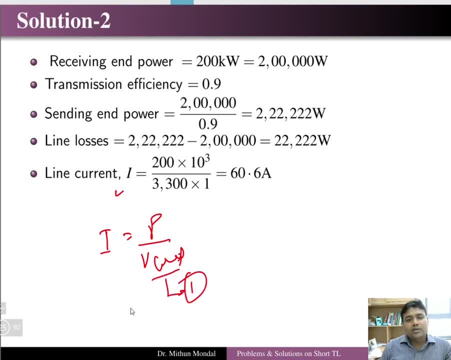 cos phi is coming to be unity, because it is a unity power factor condition and this is a single phase transmission line. So the power is given to be 200 kilowatt, The voltage is given to be 3300, cos phi is 1.. So we can easily calculate the value of the current as 60.6 ampere. Now, since, 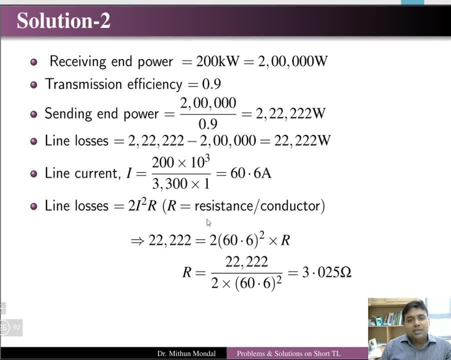 it is a single phase line and R is basically the resistance per conductor. So in single phase we know there will be two conductor, So the total line losses will be equal to 2 I square R. Now here we have been given what is the total line losses. is there? So p loss? we know, and we know what is. 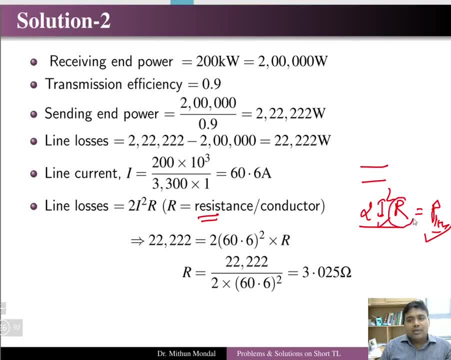 the value of the current. So we can determine what is the resistance of the line per conductor. So resistance is coming to be 3.025 on substitution. Then the length of the transmission line can be calculated from the formula: R is equal to rho l by A. So resistance is calculated, Rho is given. 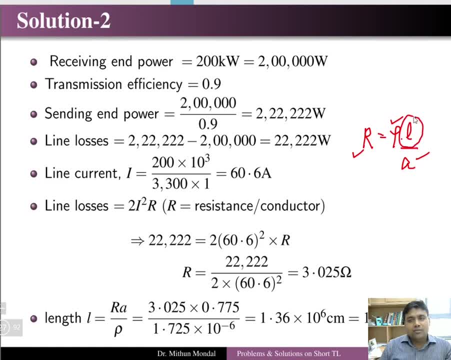 Area cross section is given So we can calculate the length of the transmission line. So length of transmission line is coming to be 13.6 kilometer. So we know that any transmission line whose length is less than 80 kilometer will come under short transmission line. so here we are getting 13.6. 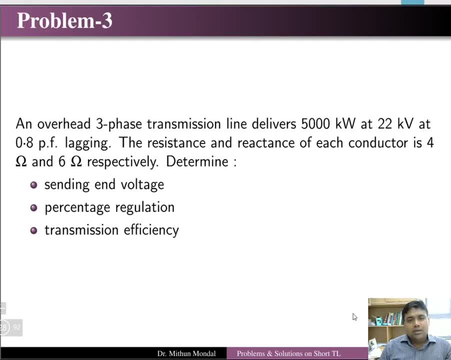 kilometer problem number three: now our calculation will start for three phase transmission line. so if you have an overhead three phase transmission line which is delivering now, whatever the load information is given to us, that is, the power at the receiving end is 5000 kilowatt and the voltage 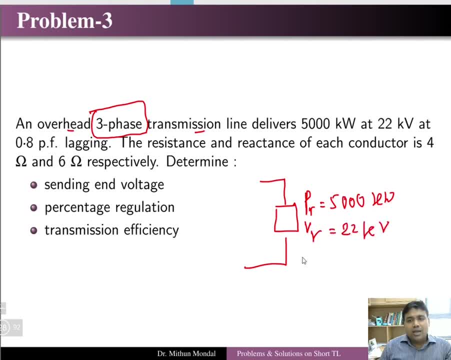 at the receiving end is 22 kV and the power factor cos phi r is given to me 0.8 power factor. now, this information is pertaining to the three phase quantities, that is, the power is three phase and this voltage is the line voltage, which was 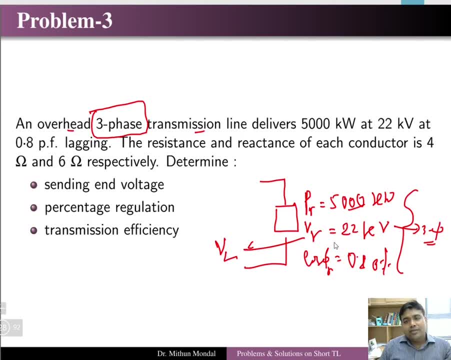 again, in single phase, these quantities was line quantity and phase quantities was equal. But however, in these, since it is a three phase system, we have to convert the three phase quantities into single phase quantities and then only we need to solve the problem. So that is the. 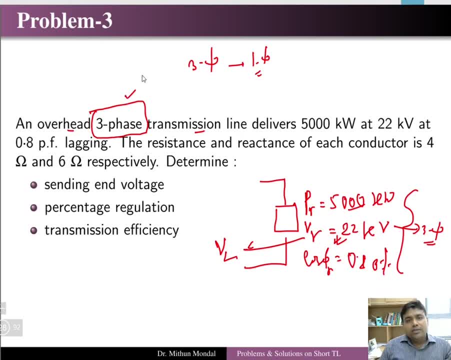 difference of a three phase system and a single phase system. Now, in a three phase system, all the quantities that is given to you, you have to convert it into single phase equivalent. The resistance and the reactance, whatever is given, it is corresponding to single phase. 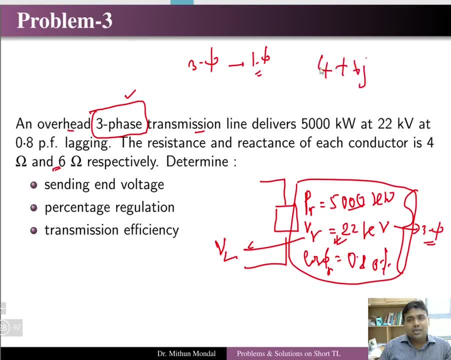 So 4 plus j6 is basically the total impedance of the single phase line. So again you have to determine the sending and voltage regulation of the line. voltage regulation and efficiency. So these are the three things we have to determine: a resistance and a voltage. So this is the three things we have to determine. 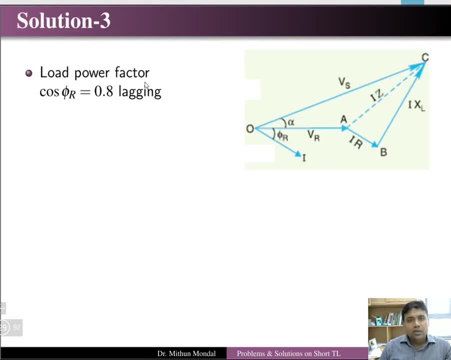 Remember this is a three phase system. So cos phi r is given to be 0.8.. So the receiving and voltage, which is again the line quantities, was given. So convert it into phase quantities by dividing it with root 3.. So you are getting 12700 volt. 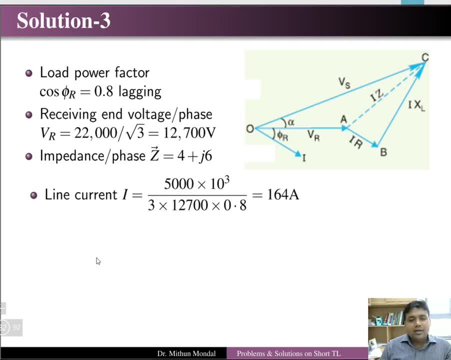 Impedance is 4 plus j6. Then the current formula will change now, because the current is equal to three times the voltage phase, current phase and cos phi. You remember, here the three term has come because it is a three phase system. So the power that is being given to you and the voltage is 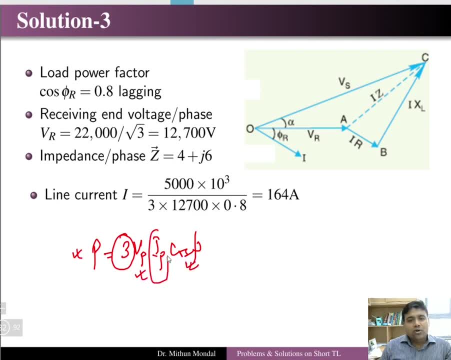 given the cos phi is given to you. So find the value of the current. So this current line current is equal to 164 ampere, which is the phase current of the system, which is the phase current of the system For a single phase equivalent circuit. Now cos phi r and sin phi r, we can obtain Then the again. 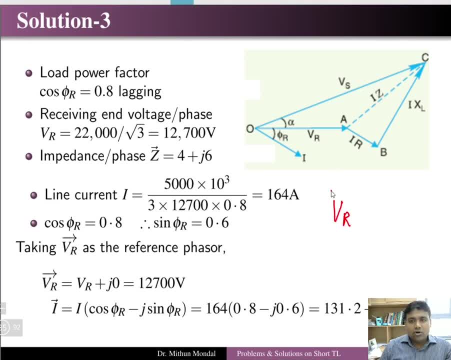 we will take the reference as the value of the Vr, So the reference is the receiving and voltage, which will have an angle, and this angle will be 0 degree, that it is there on the 0 axis, So this is a 0 degree Correct. Now the current that we have obtained is 164 ampere. that is the 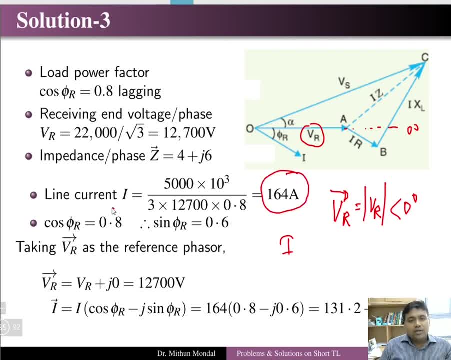 magnitude. And we have seen that the power factor cos phi r is 0.8.. So sin phi r will be 0.6.. So cos phi r minus j sin phi r will get a value of the current. Next we can calculate similarly the value of Vs. 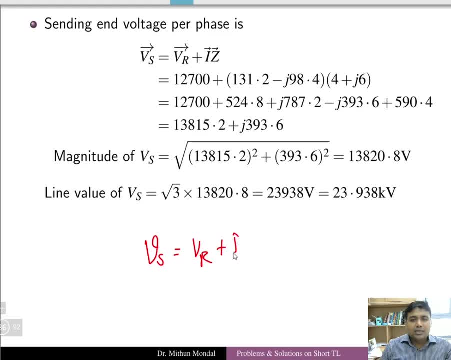 So Vs, we know that it will be equal to Vr plus the current into impedance kVr equation in the short transmission line. So we will get the value of Vs as this Magnitude will calculate under root 3.. So Vs will be equal to Vs square plus imaginary square. Similarly, whatever we have calculated in. 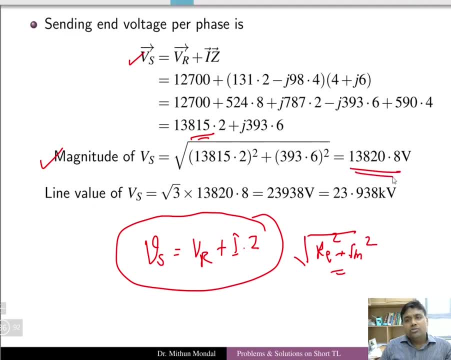 the problem number 1.. So here we are getting 138 to 0.8 volt. Now there is a little bit difference. Remember here that since it is a three phase system, we can't stick to this answer. Rather, we have to multiply with root 3 so that we convert the phase quantity into line quantity, So line. 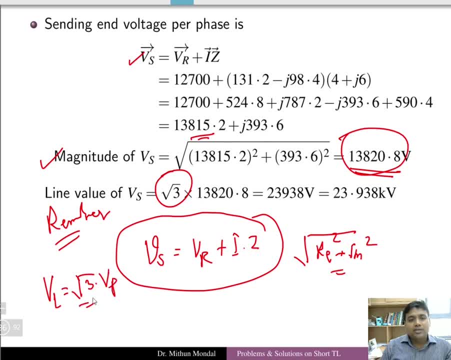 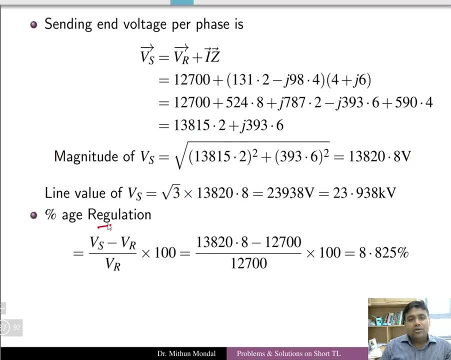 quantity is basically root 3 times the phase quantity And this gives the magnitude For the line value of the line voltage sending in. We know that the percentage regulation of the line is Sending AND voltage minus receiving, AND by receiving and voltage into 100. 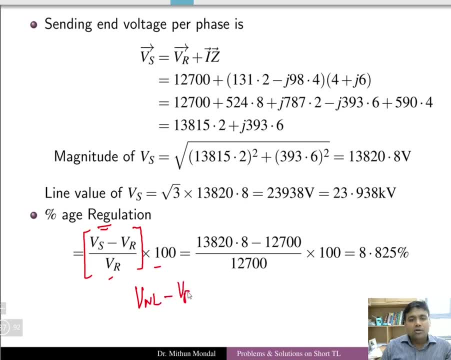 Which is nothing but the no load voltage minus full load voltage by full load voltage into hundred. So this is the voltage regulation of the line, So sending the voltage we have calculated, receiving, and a voltage is calculated So we can obtain the voltage regulation between. 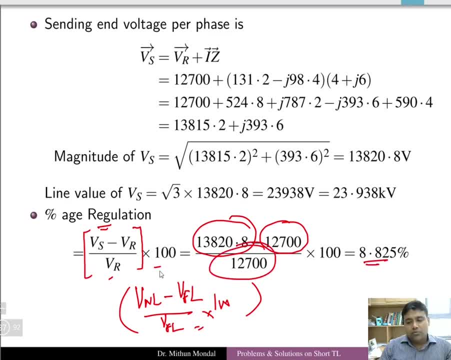 this four individual line of the line by dividing it with receiving end voltage and we have to determine the efficiency of the line. So total line losses we have to multiply it with 3 times, which was 2 times in case of single phase transmission line, and if the total resistance is given then the line losses. 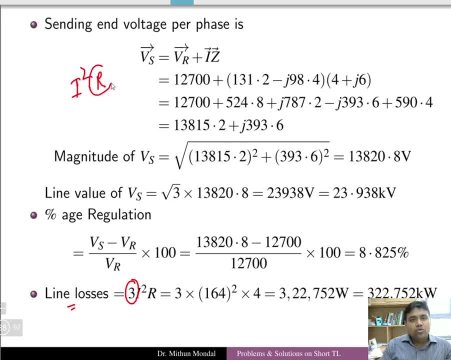 will be equal to I square R If R is the total resistance. if R is not the total resistance, then 2 I square R will be there for single phase and for three phase system it will be equal to 3 I square R. So R is basically resistance per conductor. So here we are getting 322.752. 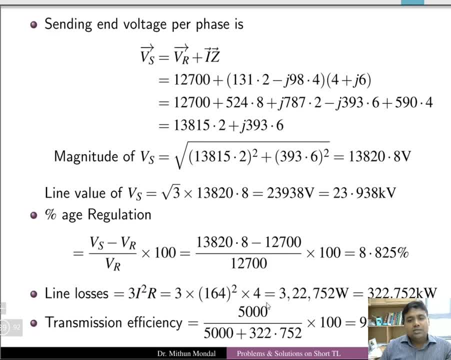 as the line losses. So transmission efficiency is power output by power input. Power input is equal to power output plus losses. So it is coming to be 93.94 percent. So problem number 1 and problem number 3.. 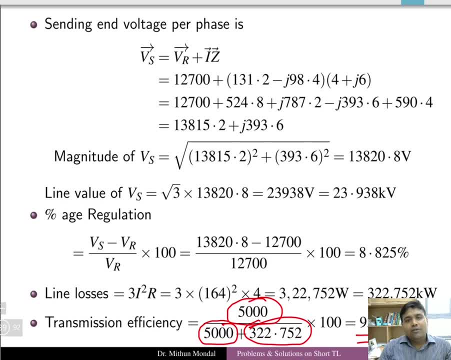 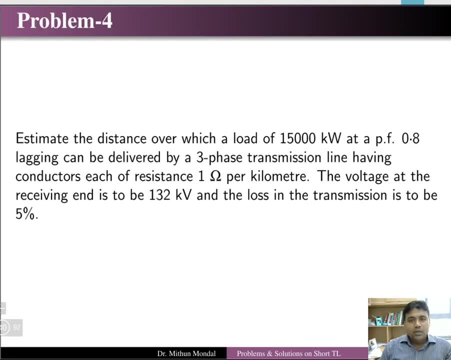 The only difference is that the problem number 1 we were solving for single phase transmission system and problem number 3 we are solving for three phase transmission system. The next problem- problem number 4- for this tutorial is the final problem is estimate the distance over which a load of 15000 kilowatt and power factor of 0.8 lagging can be delivered by 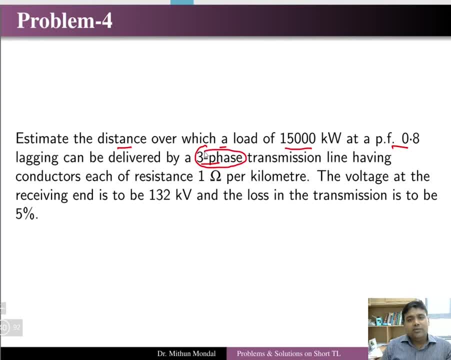 three phase transmission. Now, the special note is: this is a three phase, So these components are going to be delivered by three phase transmission. So these components are going to be delivered by three phase. So these are the three phase quantities will be the three. 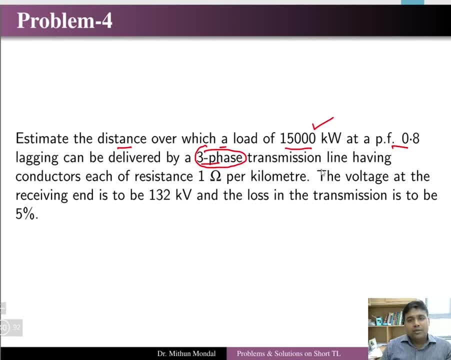 phase quantities, having having conducted each of resistance, one ohm per kilometer. So the resistance of per kilometer is one ohm. The voltage at the receiving end. So the receiving end voltage is given to be 132 kV. Now again, this voltage is the line voltage and the loss is given. 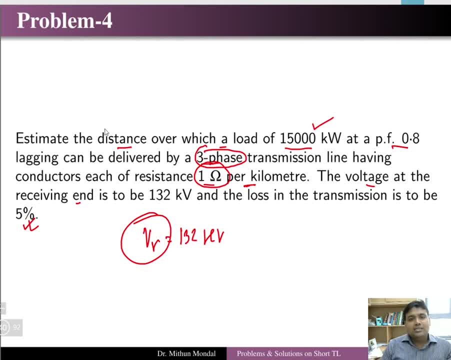 to be 5 percent. So what is the distance over which the load? So you have to calculate the total distance over which the load is given. So you have to calculate the total distance over which the load is given. So you have to calculate the total distance of the transmission line. So 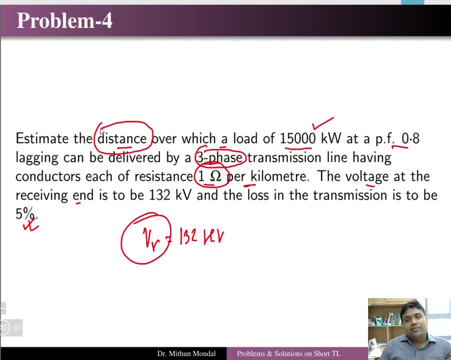 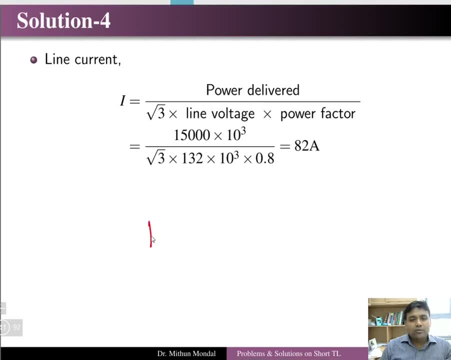 this problem is similarly to problem number two. Only difference is that here you have a three phase transmission system. So first you calculate the value of the current from the power formula. So power is basically root 3, VL, IL, cos, phi. Since it is a three phase system, you can take the line. 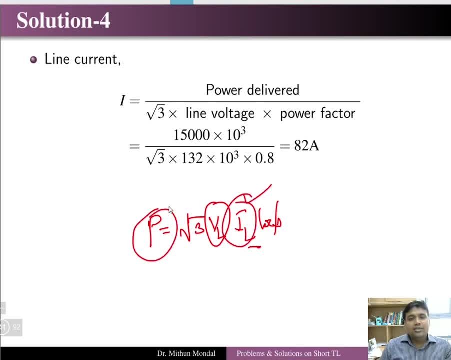